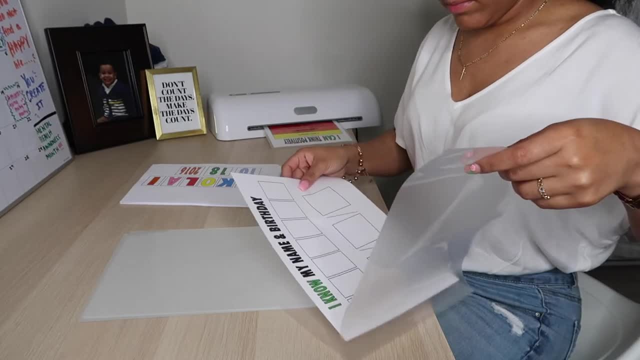 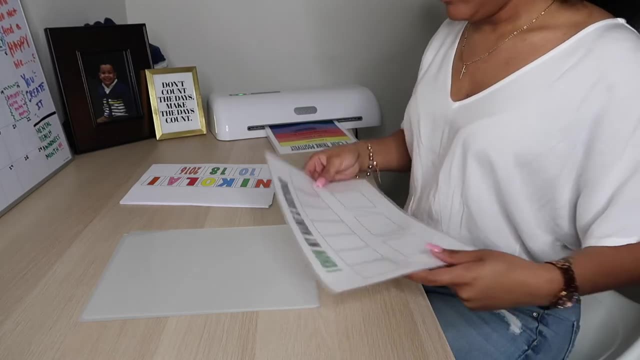 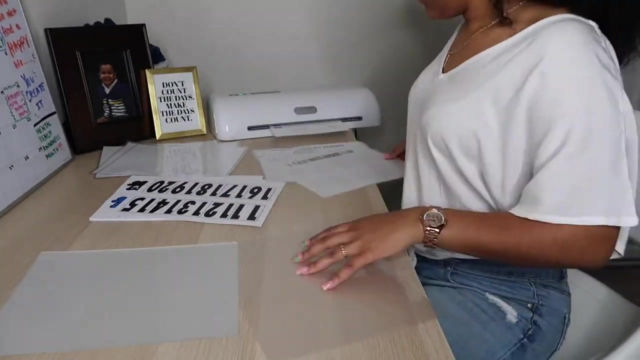 a perfectionist and make sure that they are all straight and in the middle. As you can see, here I'm multitasking. I'm inserting the pages into the pouches and I'm laminating them as I go to make this process go faster. 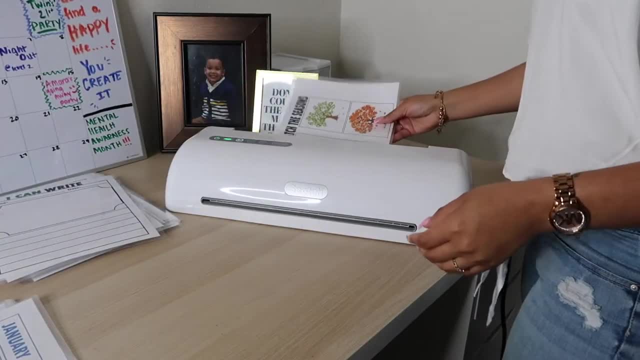 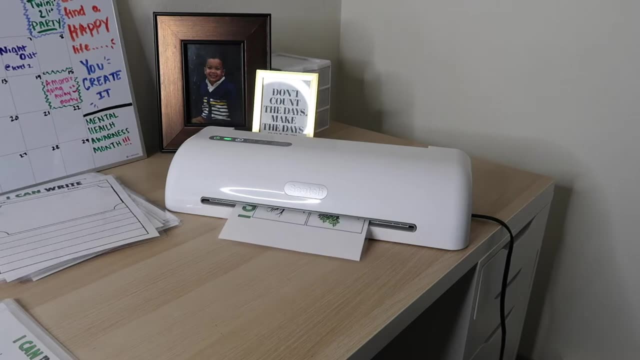 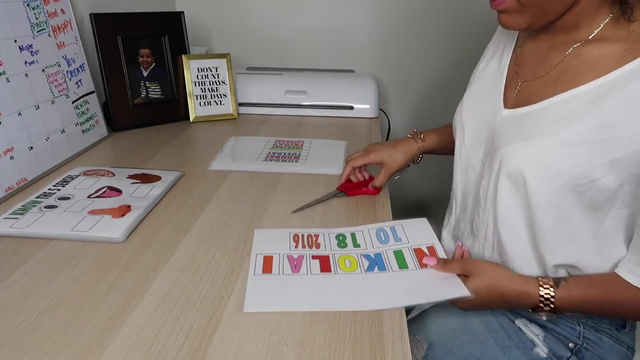 Laminating is so time consuming, y'all, because the laminator is super slow and you have to do each page individually, one at a time, So this is what takes the longest to do. After I laminate all my pages, I start cutting out the cutouts. 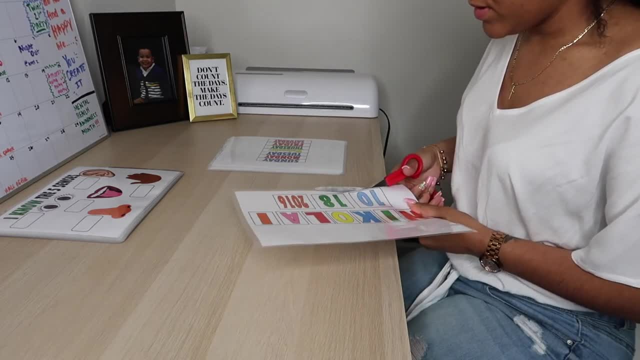 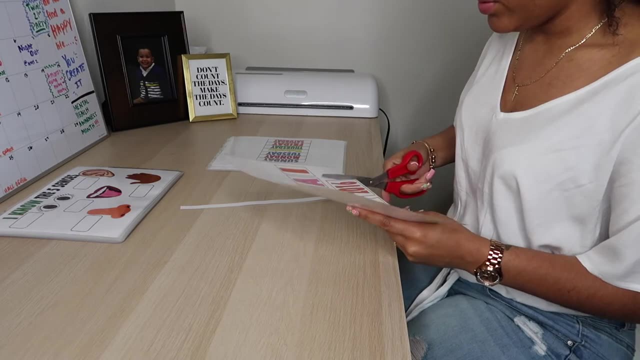 Honestly, this is one of the hardest parts for me because it's a lot of work. There's a lot of cutting involved, so my little hands and fingers be hurting so much And, as you can see here, the book is made with so much love. 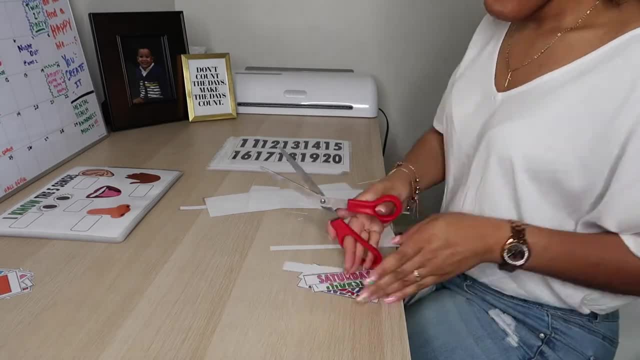 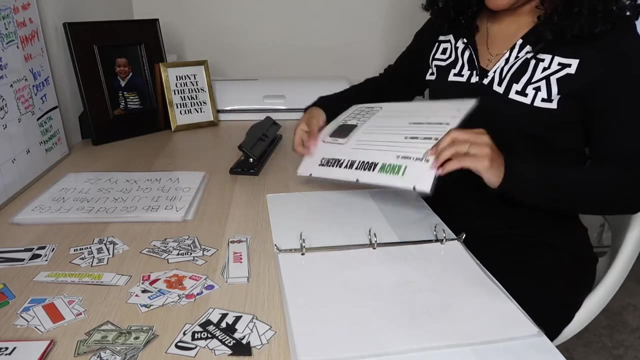 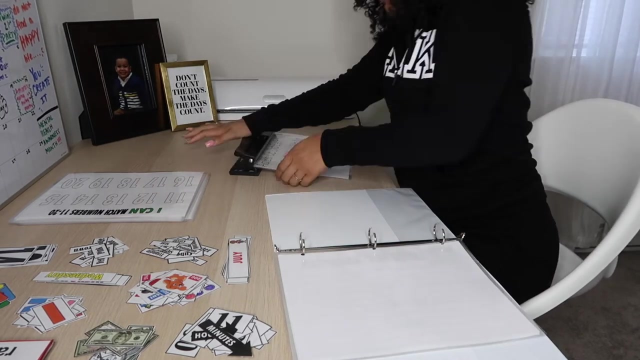 As you can tell by the outfit change, it is a new day. I couldn't finish the entire binder in one day, So here I am the next day trying to get the last parts of it together. After cutting everything, I will punch all of the pages and place them in the binder in the 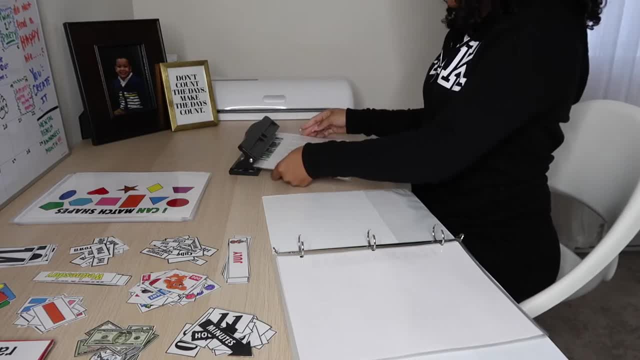 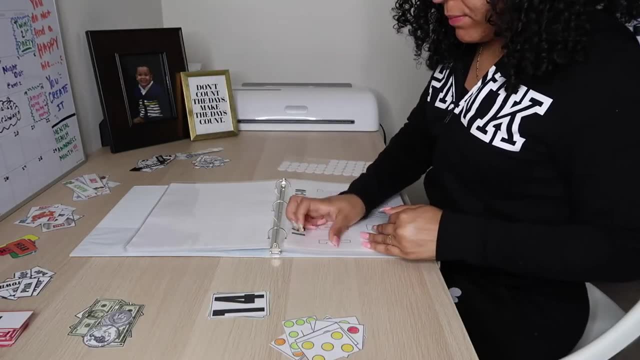 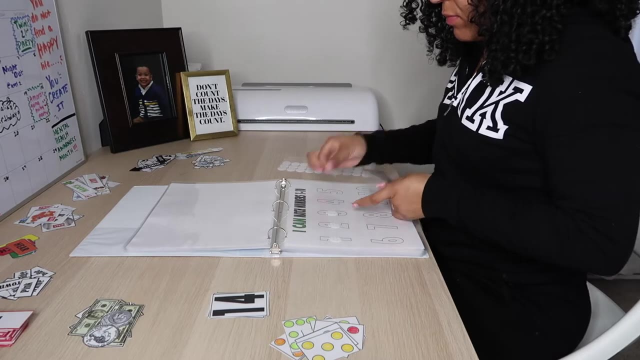 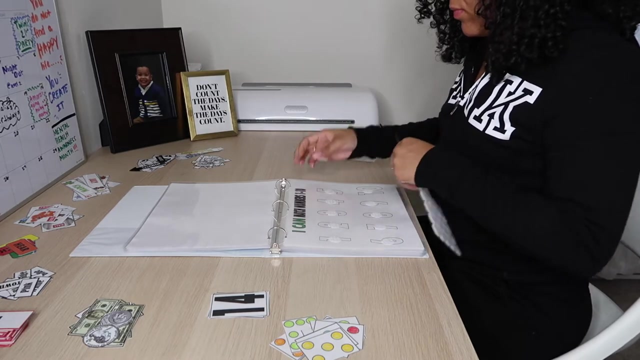 order that I want them. Lastly, I put the velcro dots wherever they're needed. After I put the first velcro dots on, I place the other one directly on top, and this helps make sure that they are placed in the right spot. so when I put the cutouts on top they're all aligned, And then I just place the 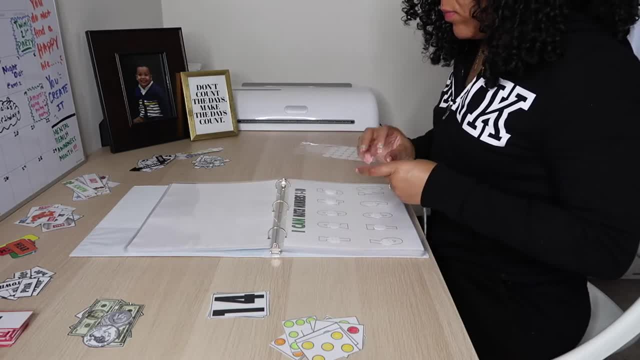 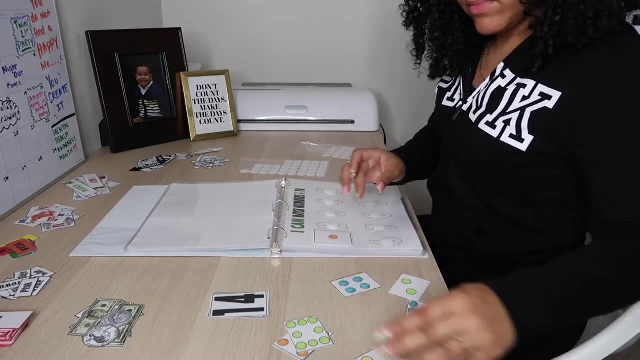 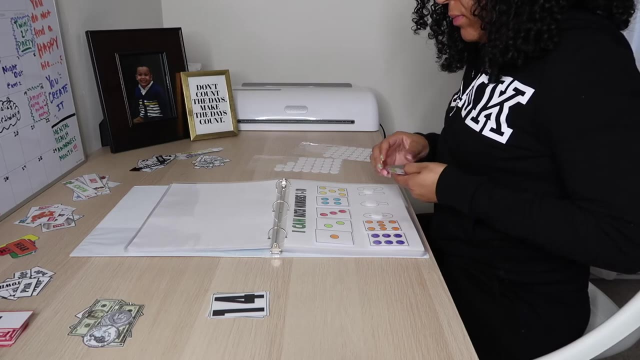 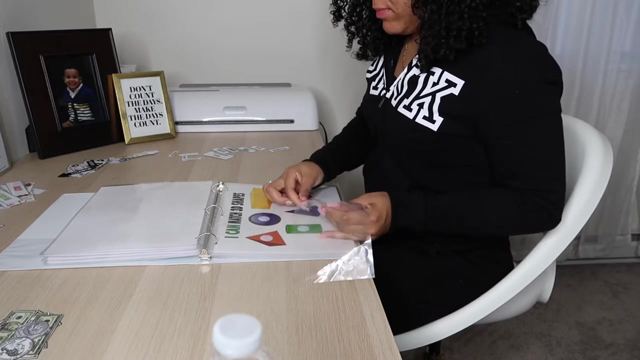 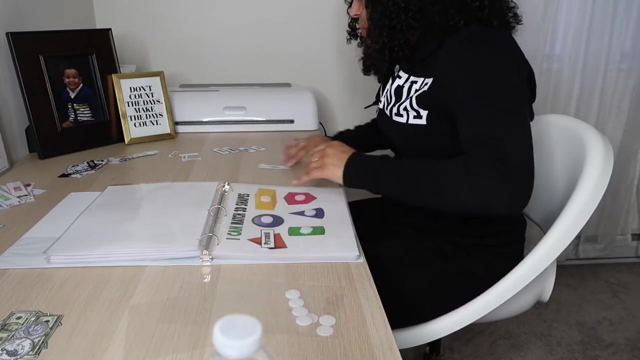 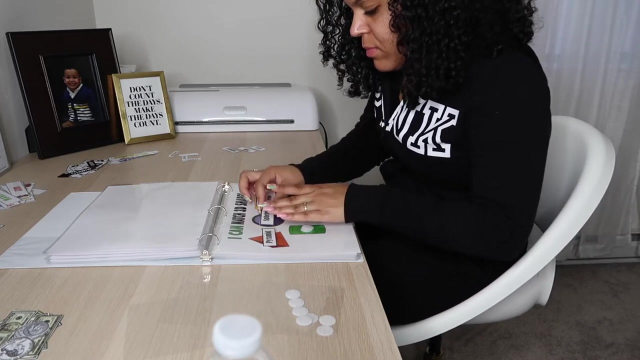 cutouts on top, and then this part is pretty self-explanatory. so just watch me do what I do, because it's hard to explain. And then I just put the velcro dots on top, and this helps make sure that they're all aligned.